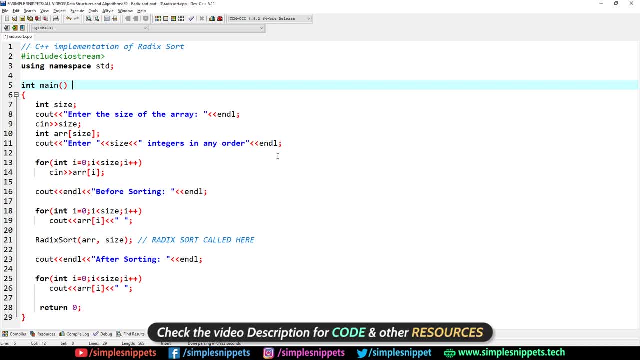 you can pause this video and type this code yourself. I highly recommend that you type this code yourself. for the best practice, open up your day c++ id or you know whatever c++ id that you're using. if you're using turbo c++, use that. if you're using any other programming, 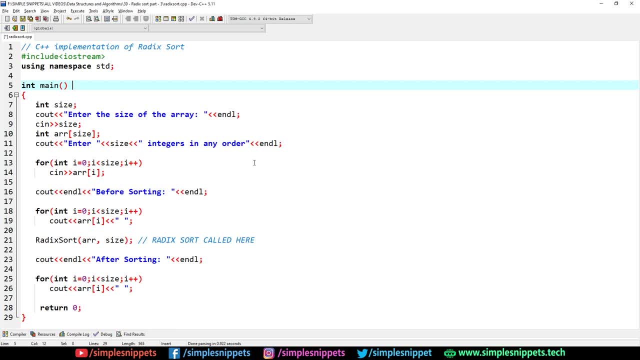 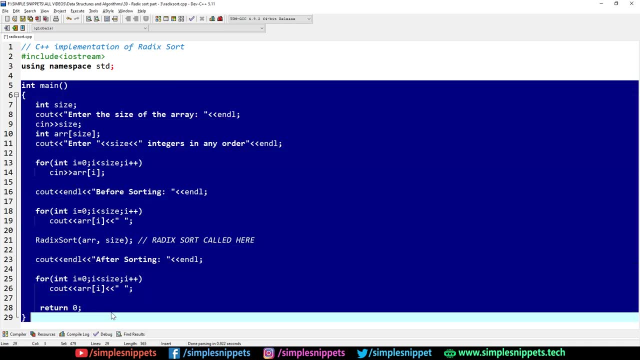 language. even then things would work, provided that the algorithm is the same. but we are using c++ and starting off, you can see, in the int main. that is the starting point of any c++ program. that is the main function. I have created an integer size. then I say: enter the size of the array. 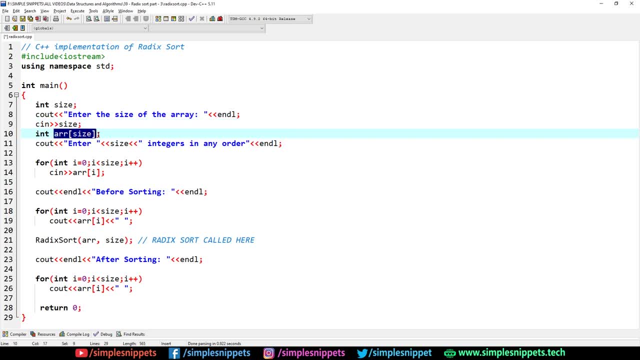 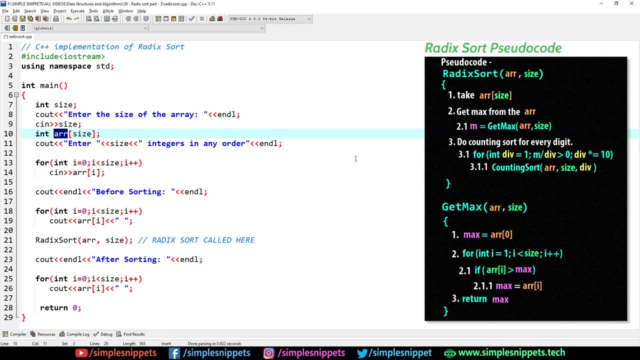 then I take in the size from the user and then I create an array of that size. okay, so array name is arr. I'll put up the sudo code. on the right hand side you can see a black screen where the code is written. According to the sudo code, the first step is to take the input array. that's what we are doing over. 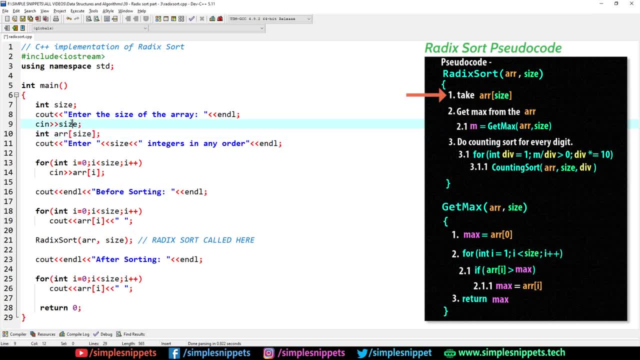 here now. if you're using turbo c++, you might not be able to create an array with a dynamic size by taking the size from the user. in that case, you can use the concept of dynamic memory allocation or you can hard code this size for simplicity purpose, after creating the array of this size. 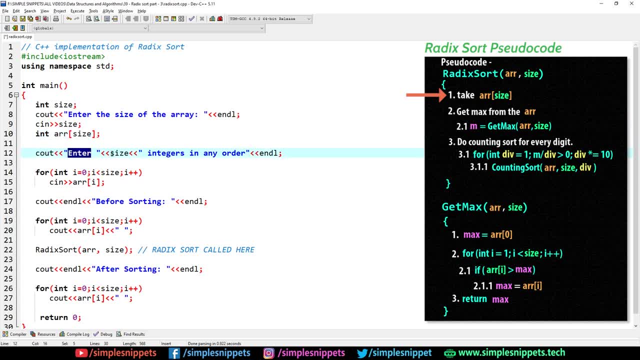 that we take from the user. I say cout: enter size, number of integers in any order. so if I enter the text that will be printed on the cmd would be: enter five integers in any order. so this is again step one, only in the sudo code that is taking the input, taking the input array. so this for loop. 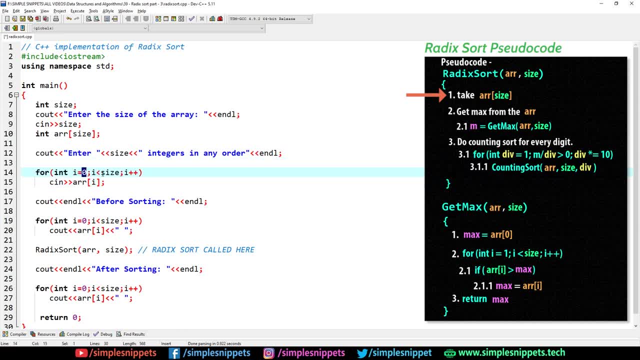 basically takes the input array starts from i equals to zero to i less than size, and then c in arr of i. so we are taking every element in the array from the user and you don't need brackets when we have only one statement in the for loop. so that's why we don't have curly braces, basically. 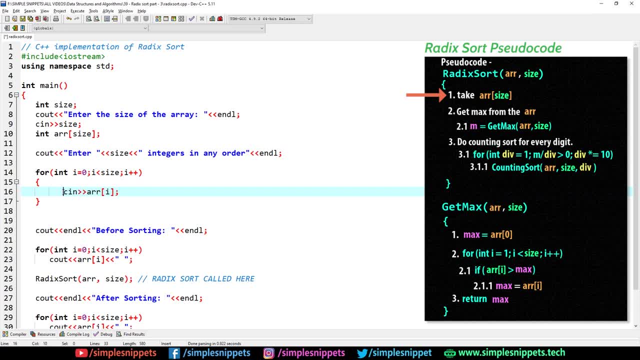 but if it is confusing- here are the curly braces- then I say cout, I say before sorting, I again use a for loop, and this time again from zero to size. I'm just printing out the array. this is before sorting. okay, after that I'm calling a function, user defined function, radix, sort which. 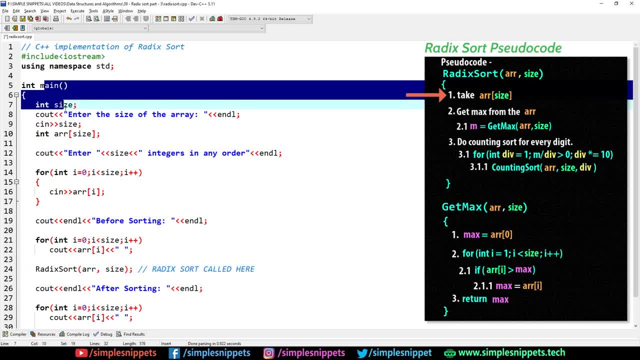 we still have to create, so we'll create that over here. this is just the main function in that I'm passing this array that we've created. so if you see the pseudo code of radix sort, the two parameters are the array and the size of the array. so radix sort is called here. we still. 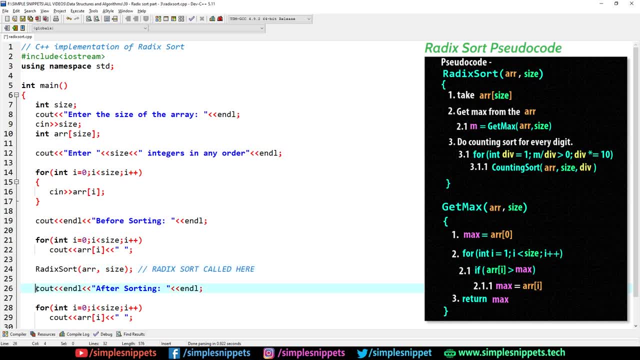 have to create this function. that we'll do in a minute. after that, obviously, the array will be sorted. when you're passing an array as an argument in c++ it is passed by address and not by value, so whatever changes that are made inside this function on this array will be actually reflected. 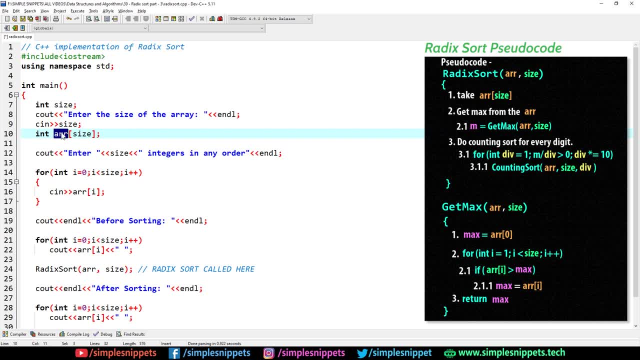 back onto our original array also, right. so I hope you know what is the concept of pass by value, pass by address, pass by reference. if not, I have a very good video explaining these three concepts. I'll link that in the video description. you can check out the c c++ playlist as well. but yeah, after. 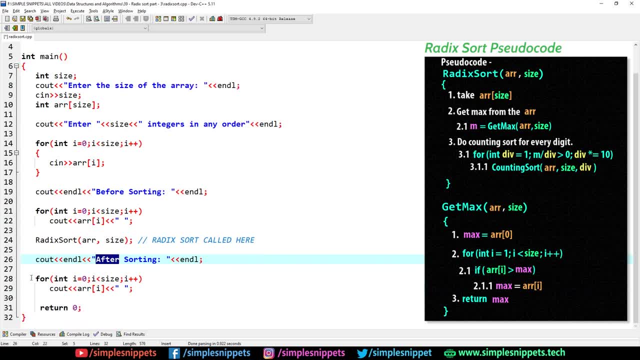 the radix sort is called, again I print after sorting and then again I use a for loop. again I output all the array elements, but this time they would be in sorted manner, and then last statement returns zero. so this is the end main. I did not type it from scratch, because then we 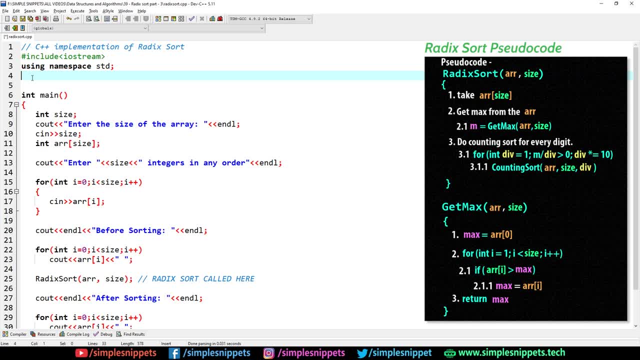 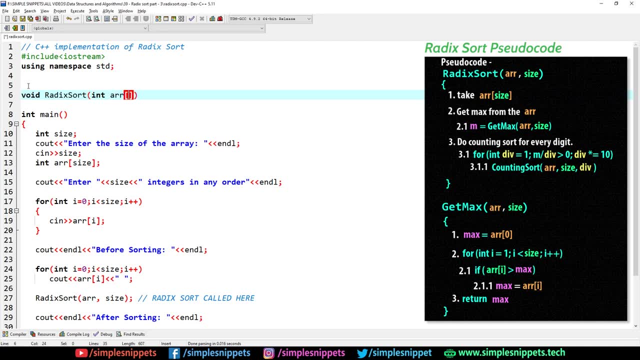 would be wasting time. but now let's get started with creating the radix sort function. so I'll just say void radix sort And it is going to take integer array. So I'm going to say int ARR, with opening and closing square brackets to denote that it is an array And it is also. 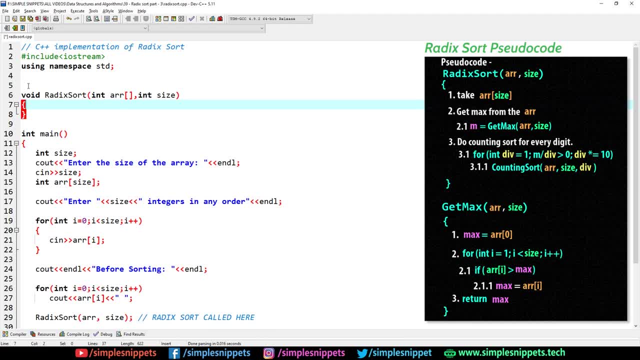 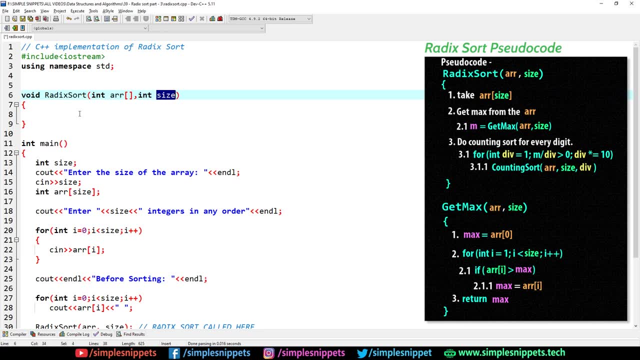 going to take integer size as an argument. So that is exactly what we are passing: ARR and size. So this ARR and size are variables which are created, just for you know, this function inside this function. So even though the names are same, they are two separate. 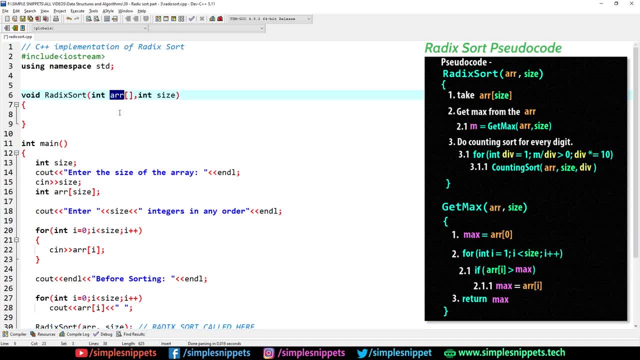 variables And, as I mentioned, this array is going to be passed by address. So when you're passing an array in a function, you don't need to have square brackets, but when you're creating that function, this is the user defined function. that time we have to. 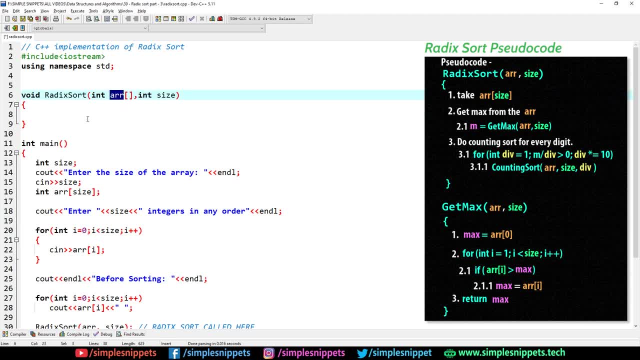 mention the square brackets to denote that this is the array that is going to be passed. Okay, Now, if you see the step two in the pseudocode, the next step is to get the maximum from this array. So I'm going to say int m is equal to get Max. Again, I'm gonna pass. 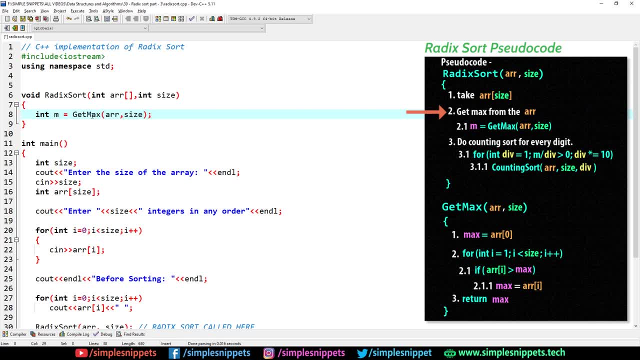 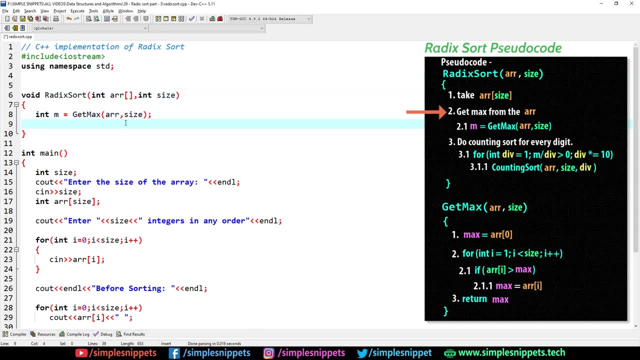 this array and the size of that area. now again, we have to create this get max function. so we'll create it in a minute. but let's complete the radix sort function. after we get this m, we have a for loop. we say for in div is: 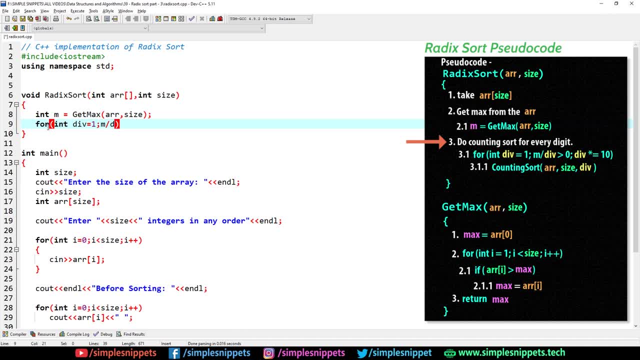 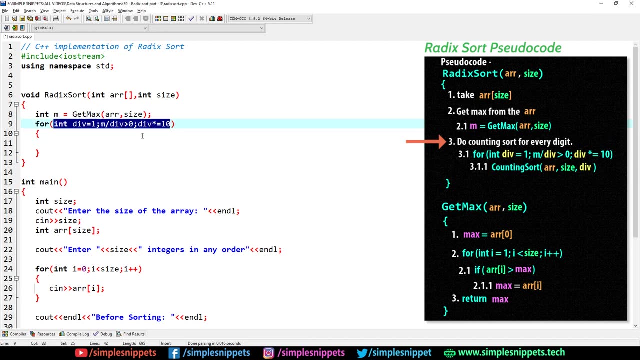 equal to 1 m by div should be greater than 0 and the increment is div star equal to 10. now we've already discussed in detail about these conditions in the previous tutorial, when we saw the pseudo code, so i'm not going to repeat it over and over again, just watch. 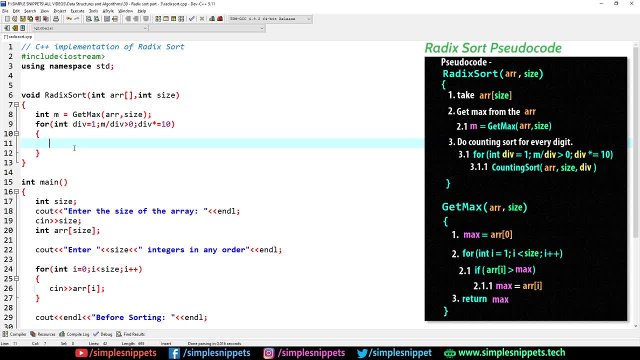 that that is very important to understand the behind the scenes working. this is just converting the pseudo code into c++ code, but this for loop condition is basically used to call counting sort multiple times, and the number of times counting sort is called is going to be equal to the number of digits that the maximum number has in the array. that 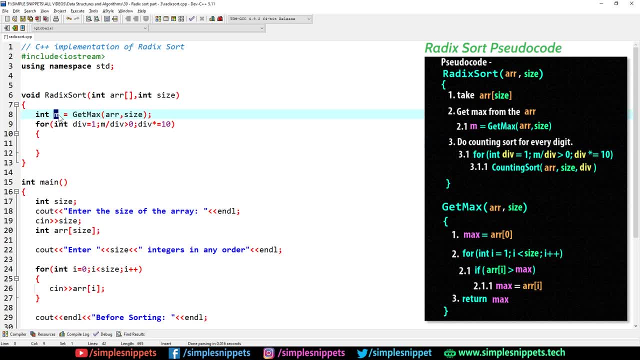 is why we call the get max over here. we have that in this m number. so at every iteration of the for loop the m will be divided by div. first time div will be 1, second time it would be 10, and the third time it will be 100, and so on and so forth. so this will happen depending 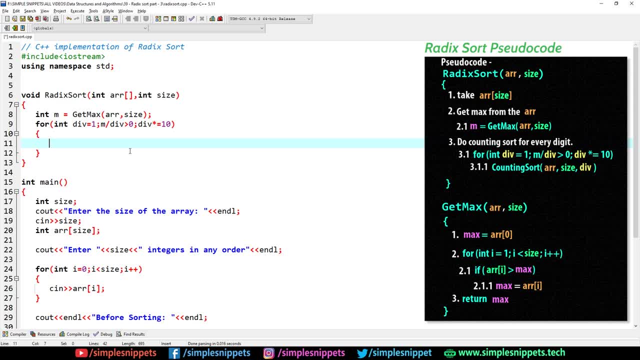 upon the number of digits in the maximum number in the array and then inside the for loop we call counting sort. we pass the array size and div. okay, so that is exactly what we have in the pseudo code as well. so this is the complete radix sort function, but we still have to create the get max and the counting. 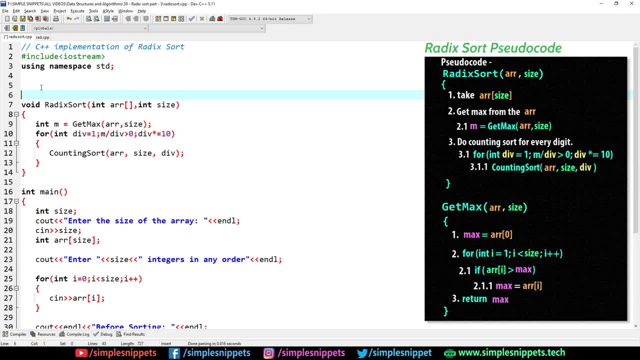 sort function separately. so let's first create get max. so get max, you can see, is on the rhs, which means that it is returning integer value, because on the lhs we have an integer variable. so i have to say int- get max and of course it is going to take an integer array, so int. 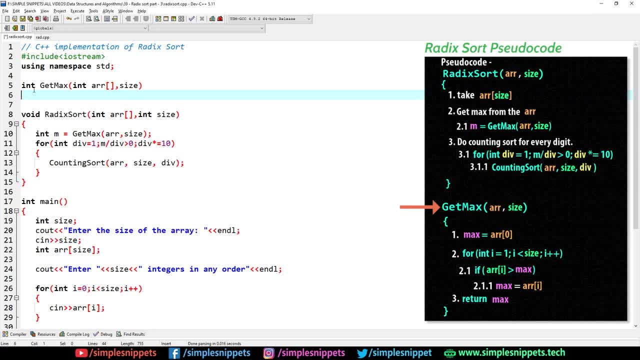 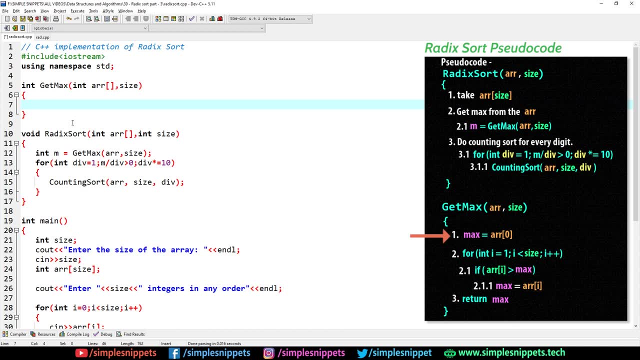 arr comma size, because that is what we are passing over here. right, the array size is the array and the size. now the first step in the get max pseudo code, as you can see on the right hand side, is to declare a max variable and take the first element from the. 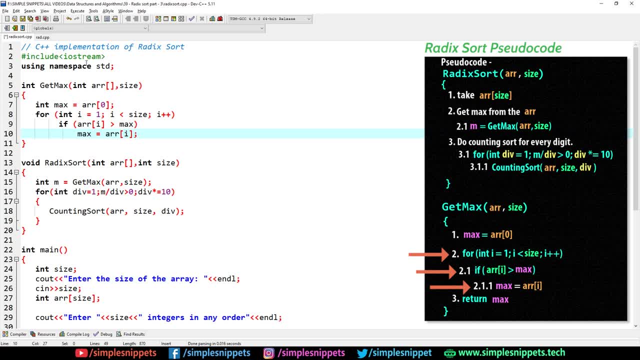 array and store it over there. after that we call a for loop. we say for int i equals to one, i less than size. so we are iterating from one till the size, that is one less than the size, and i plus plus. and inside that we have a if condition. we say if arr is greater than 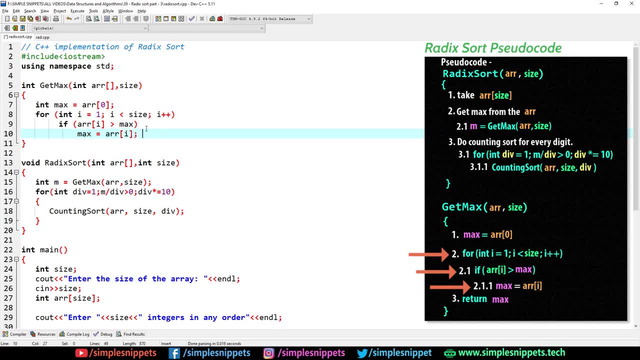 the max value, then the new max value is going to be the arr of i and so when we do that- okay, so I've not used brackets anywhere, but if I were to use brackets, this is how it would look like. if we have only one statement inside the if block or for loop, then we don't really need to. 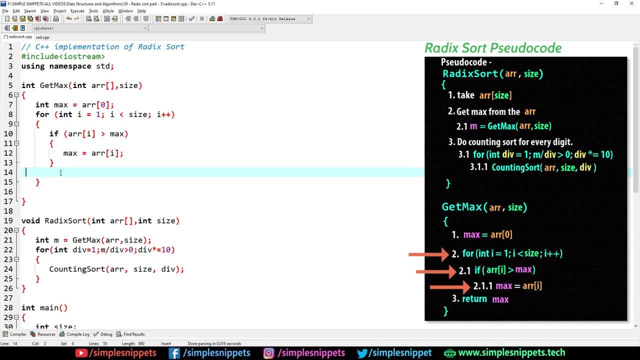 use the brackets. we can do away with the brackets, but sometimes it gets a little confusing. so yeah, this is how it would look like with brackets. and lastly, we have to say return max. okay, so this is the get max function. so this get max is called over here. we will get the maximum over here, and 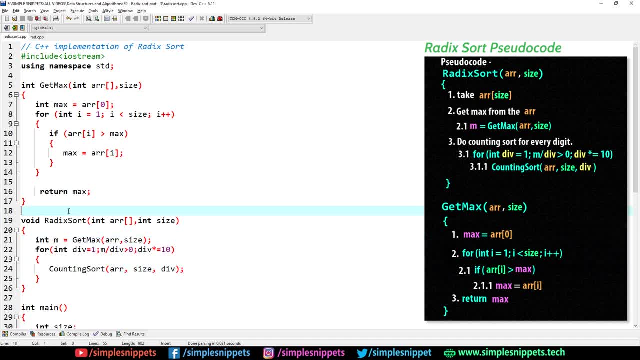 then we will go inside the for loop and now we have to create the counting sort function as well. so we've already covered counting sort, the working of counting sort and the implementation of counting sort in a separate tutorial in this playlist itself, so I'm not going to go ahead and type it. 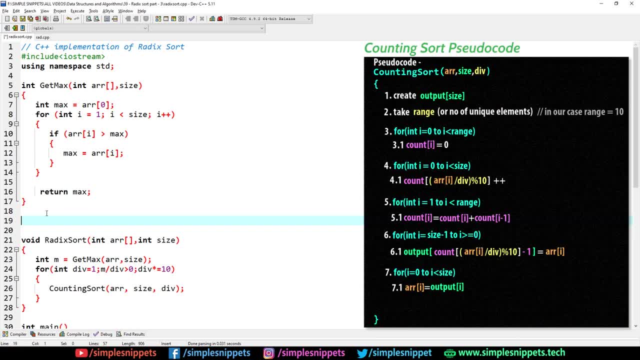 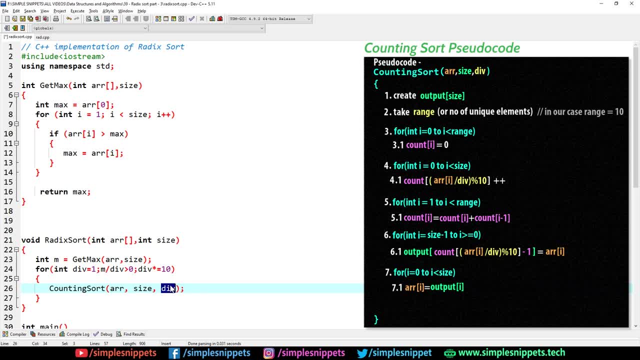 is one digit in the multi-digit integer in every iteration. so in first iteration we're going to get the units place in. second, we are going to get the tenths place in. third, we are going to get the hundreds place for every element, depending upon how many you know. maximum number of digits we 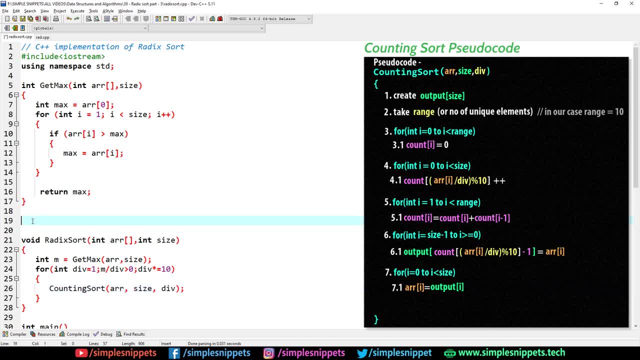 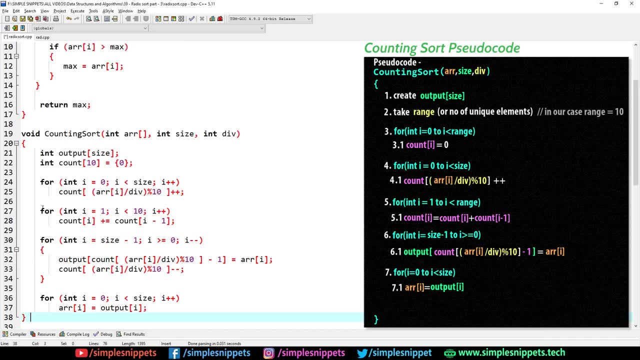 have in one particular in the maximum number. so I'll just paste the code of the counting sort function over here and then we'll go line by line and I'll also show the pseudocode on the right. so this is the counting sort function. it is taking an array. 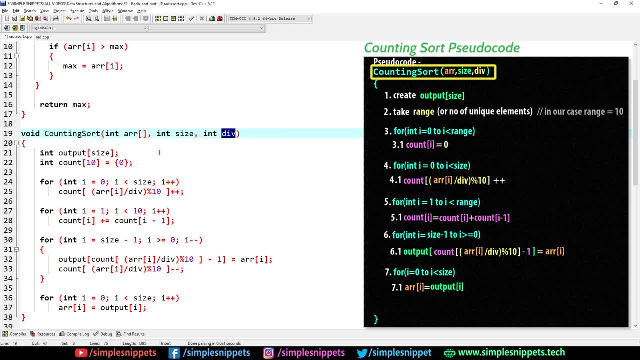 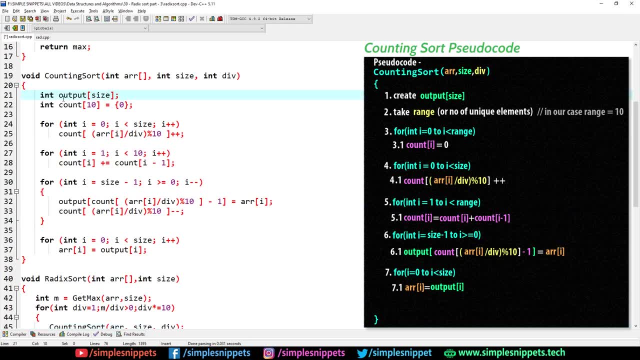 it is taking the size of the array and it is taking that div variable. so in the radix sort you can see counting sort is called. we are passing array size and div. so coming to the counting sort now, step one is to create the output. so we are creating output array. 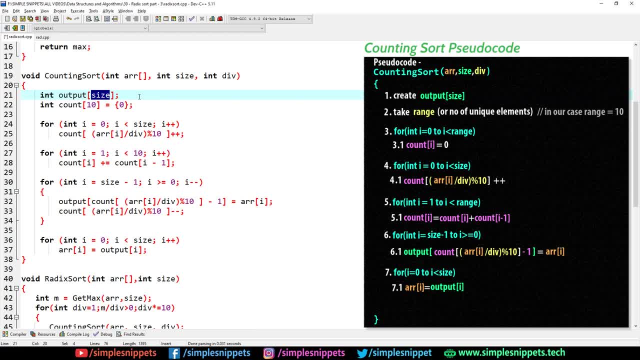 of the same size as the input array. now the range obviously is going to be 10. we've discussed why it is going to be 10, because in decimal number system we have only 10 unique elements or 10 digits, that is, from 0 to 9, and since we are applying counting sort on single digit, 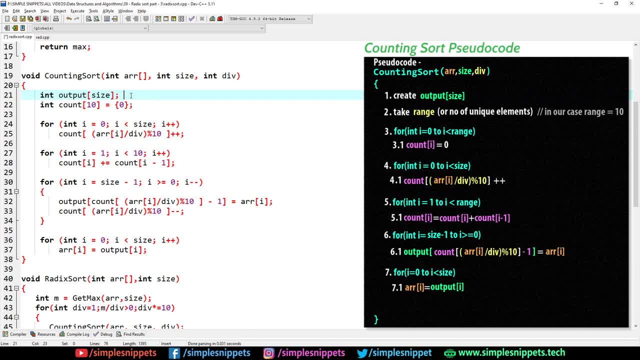 of every number in the array. the range obviously is going to go from 0 to 9 only. hence we have to create a count array of size 10 and initialize it initially to 0. so this syntax basically makes all elements in the count array 0, or you can use a for loop also in the pseudocode. 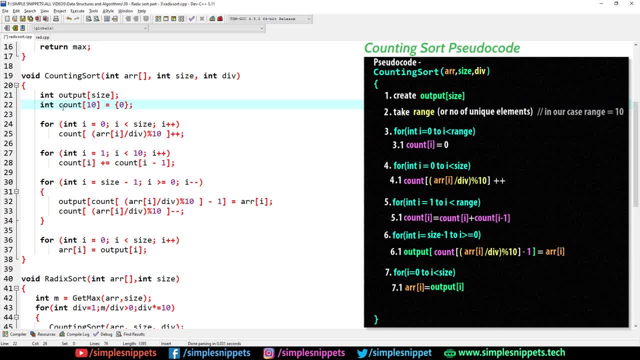 you can see in step number 3 and 3.1, we are using a for loop 0. or you can use a for loop also in the pseudocode. you can see in step number 3 and 3.1, we are using a for loop. 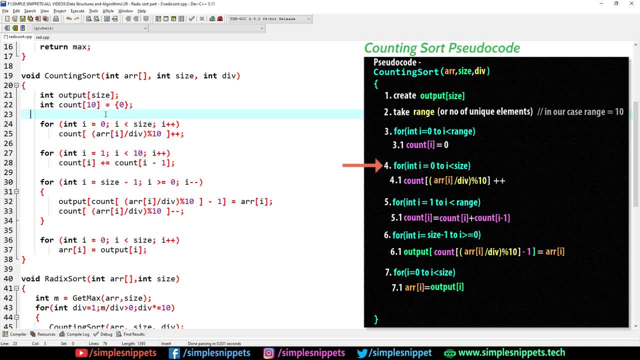 but you can use this syntax also. moving on for the 4 and 4.1 step, we are taking a count of all the elements and the count is basically taken by taking one single digit of the number starting from the lsb. so for the first iteration we are going to take the units place, if it. 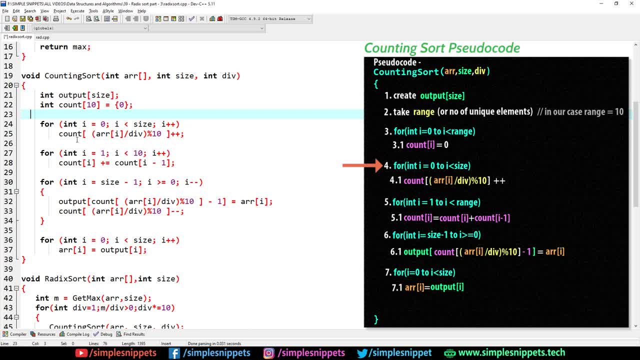 is a 0, we will come in the array, in the count array, at the 0 location, so count of 0 will become plus, plus. if the units place of the number in the input array is, let's say, 5, then in the count array at the 5 index position we will come and we will say plus, plus. so 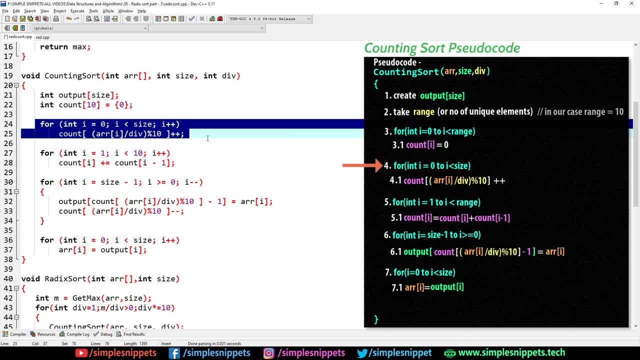 that is what is happening in this for loop in step number 4 and 4.1. so that is this for loop. again, i have not used brackets because you only have one statement. then the next for loop is for taking the cumulative count, so count of i plus equal to count of i minus. 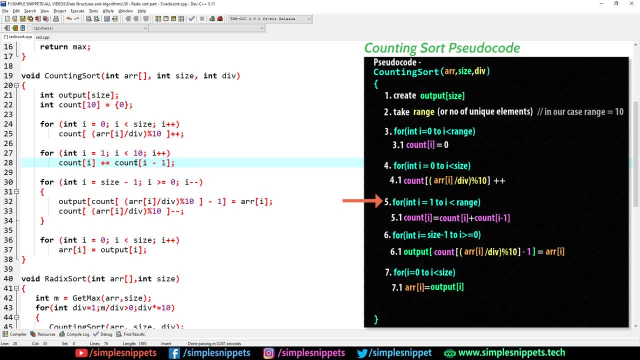 1. so that would be: count of i is equal to count of i plus count of i minus 1. that is exactly what we have in step number 5 and 5.1. now step number 6 and 6.1 we are going. 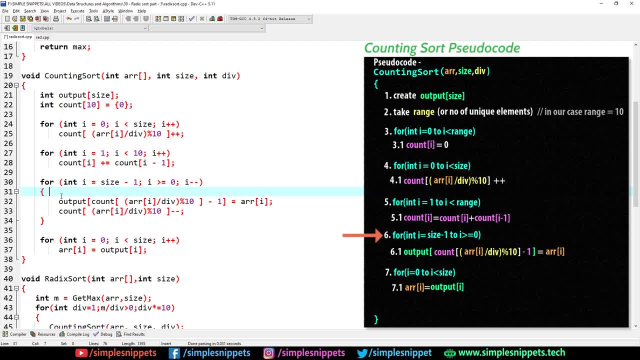 to do is that we have the following for loop: step number 6 and 6.1 in the pseudo code is basically that for loop where we are taking one element from the input array and we are putting it in the output array at a particular position, using this newly calculated count. 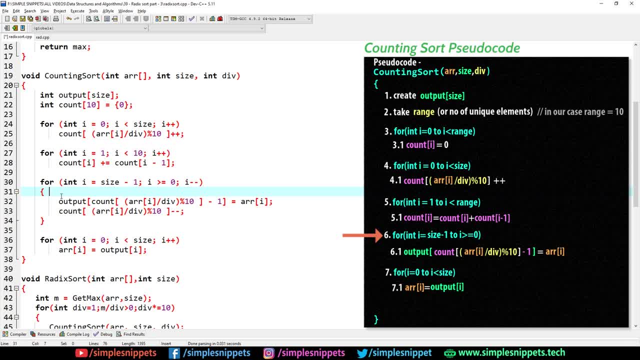 array, which is the cumulative count, which is storing the exact positions, and that is done using this expression. and then we have to also decrement the count. so we are saying count of, again using that same expression. we go to that index position and say minus, minus. so this mapping we've thoroughly discussed in the previous video where we discussed the 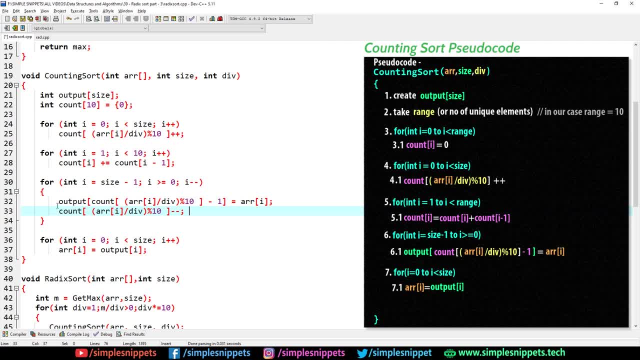 pseudo code and we are using this for loop, so we are taking one element from the input code. please watch that for better understanding here. you might not understand it if you try to. you know dry run it. you can even dry run it over here, but that's where we already have dry run it. so 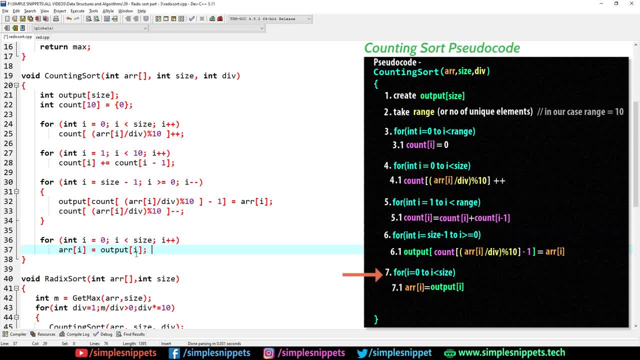 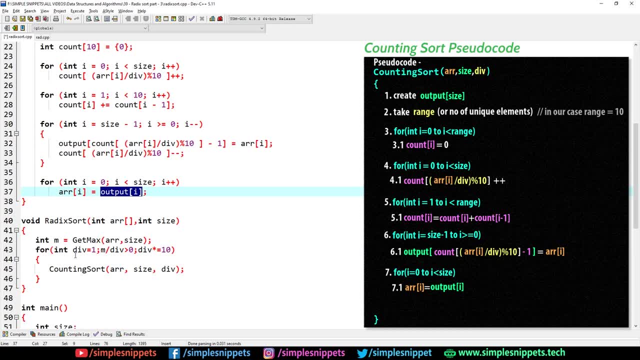 you'll understand that much better. and this last for loop is again taking the output array and transferring all the elements from the output array to the input array. so, yeah, this is the entire code. i'm obviously going to be sharing this entire code, along with the theory, along. 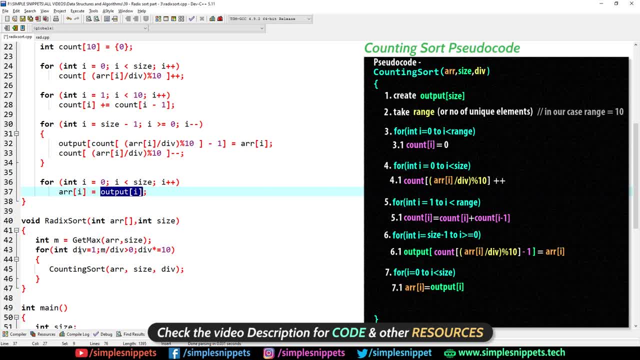 with all the details for radix, sort, sorting, whatever things we've discussed in the previous three videos of this radix or topic. i'm going to be sharing all of that on our official website so you'll see that link in the video description. if you're preparing answers, if you're, you know. 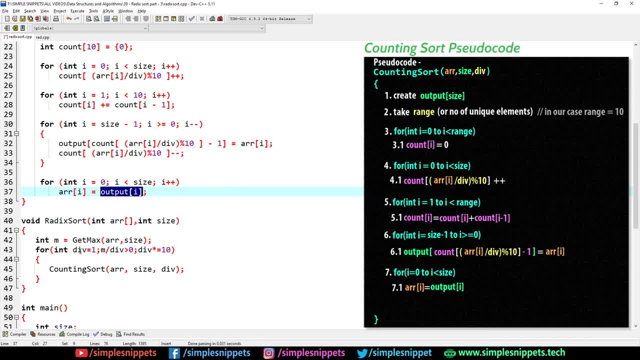 writing the code. you want to copy paste the code. you want to prepare your answers. go through that article. that will have all the information and we've pretty much done with the code. let's save this and try to compile and run. i hope we don't get any errors. and we did get an error, okay, so 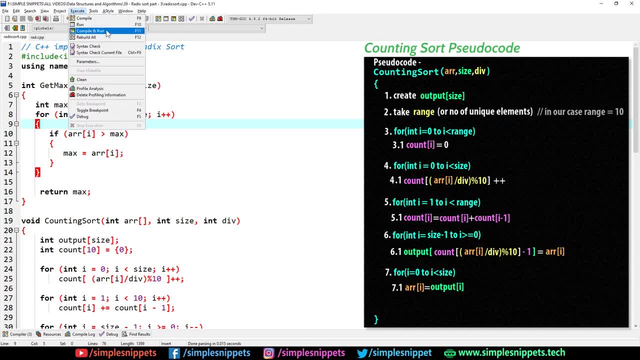 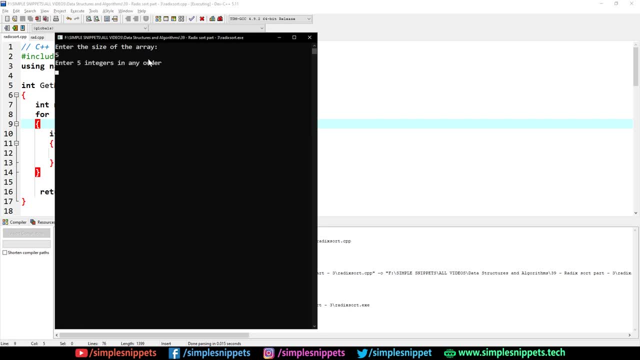 this has to be int size and i think we are good to go. okay, our code is done, so let's go ahead and run it and we'll see what happens next. so let's go ahead and running. fine, let's enter the size of the array. let's say we have an array of size five. now we 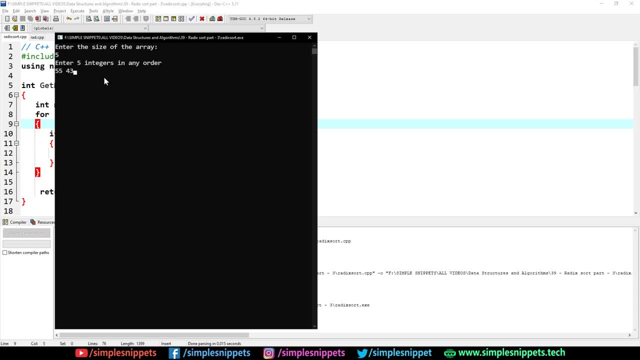 have to enter any integers in any order. so i'm going to say 55, 43, 1, 6, 7, 8 and 5. so 1, 2, 3, 4 and 5. so the maximum number over here is 6, 7, 8. it has three digits, so counting sort will be called three. 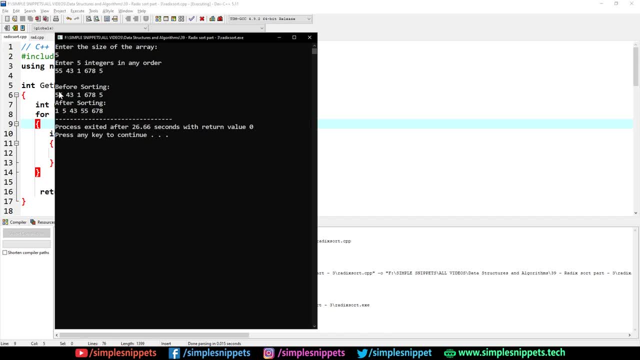 times when i hit enter. so there you go. before sorting i'm getting the same array: 55, 43, 1, 6, 7, 8 and 5. but after sorting you can see i'm getting 1, 5, 43, 55 and 6, 7, 8. so this is properly sorted, which means that our 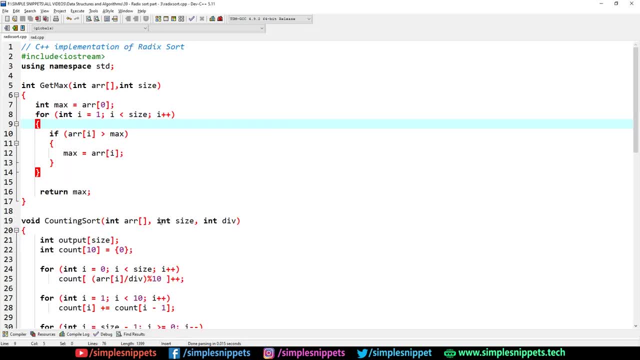 radix sort is working perfectly fine. okay, so that's it for this video, guys. this was the implementation, the practical aspect of radix sort, where we wrote a c plus plus program to implement radix sort, which essentially uses counting sort multiple times. so that's it for this video, guys, if you've understood. 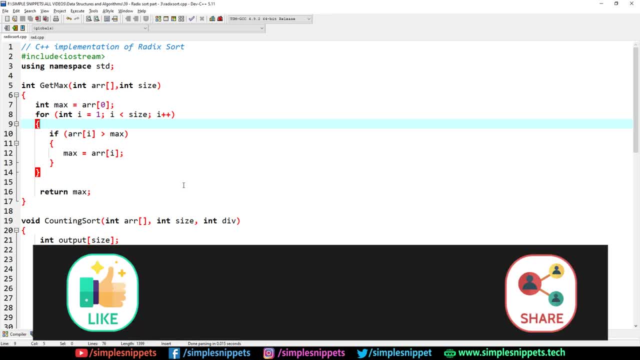 this code. if you like this video, please give it a thumbs up. do share this video. in fact, do share this entire dsa course, dsa playlist with your friends. this is a very fundamental topic. there are a lot of many other topics inside this course. let me know in the comments how. 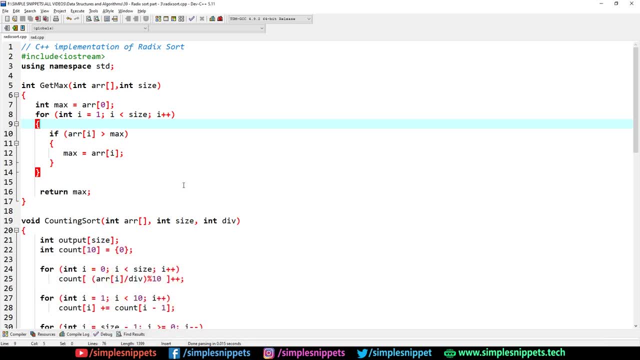 this video was, and i'll see you guys in the next one- peace. 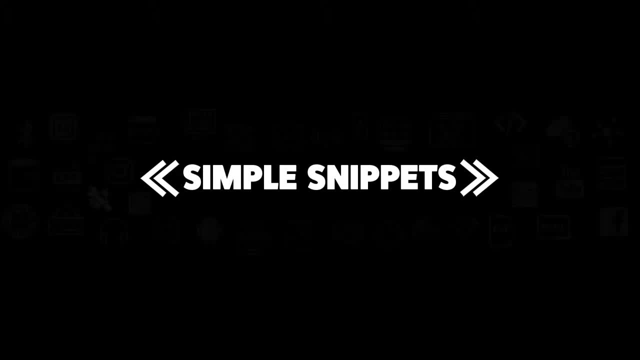 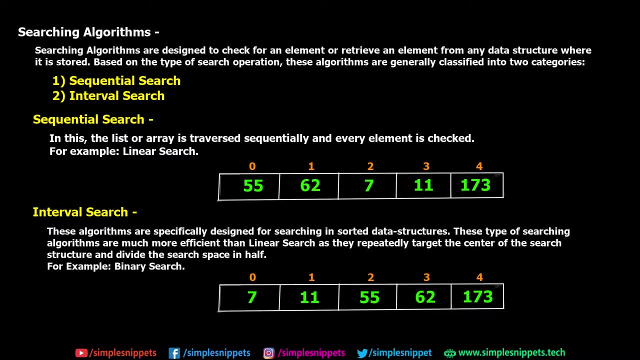 Yo, what's going on guys? Tanmay here for Simple Snippets and welcome back to another video tutorial on Data Structures and Algorithms, and today's topic is going to be searching algorithms, especially the sequential search. Before we start off with the topic, a quick 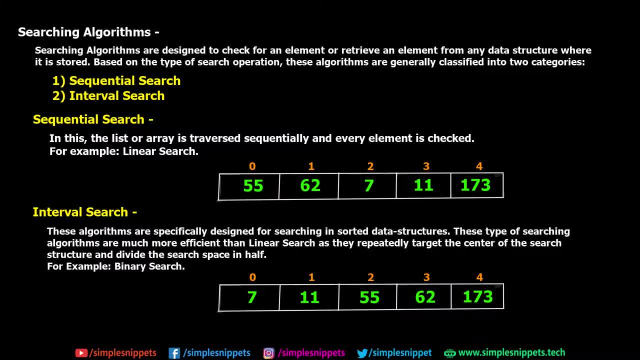 note: I have a complete Data Structures and Algorithms playlist. If you are new on this channel, if you are watching this video for the first time, check out this entire playlist. There are a lot of topics covered under Data Structures and Algorithms, and more are frequently.